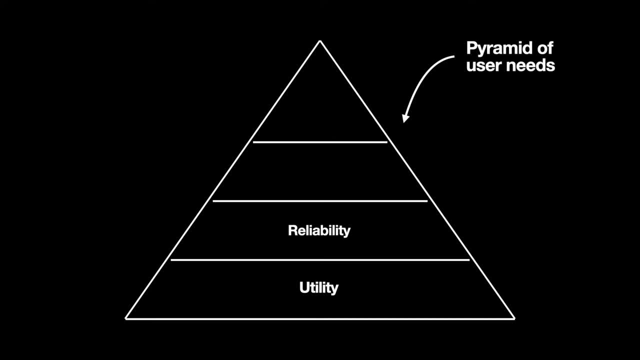 Any unexpected problems that users face as they interact with your product will make them doubt whether they can rely on it in the long term. Next comes usability: Users' ability to use a product. It's not enough for a product to be reliable: It also should be usable. 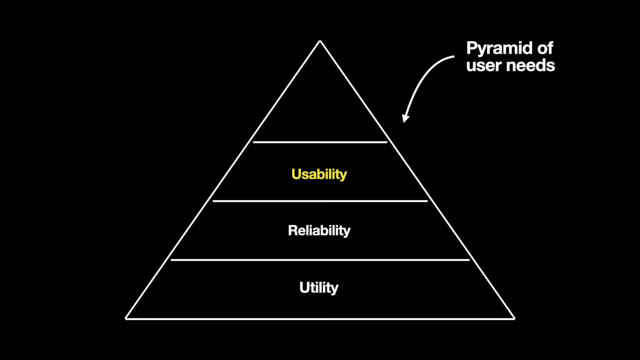 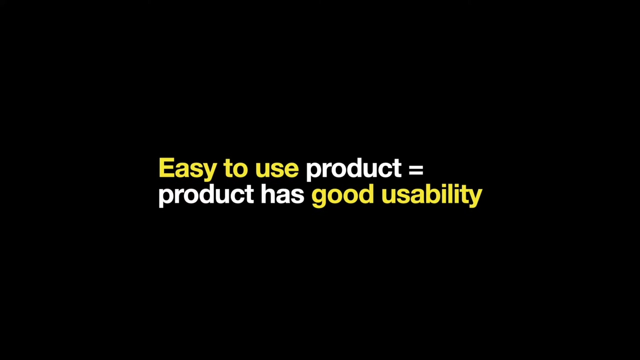 When we try to improve usability, we aim to find and remove any barriers that prevent an efficient human-computer interaction. Finally, pleasurability: Pleasurability refers to any positive emotional response that users receive from interacting with a product. When we conduct heuristic evaluation, we aim to identify usability flaws so that the team can design an easy-to-use product. 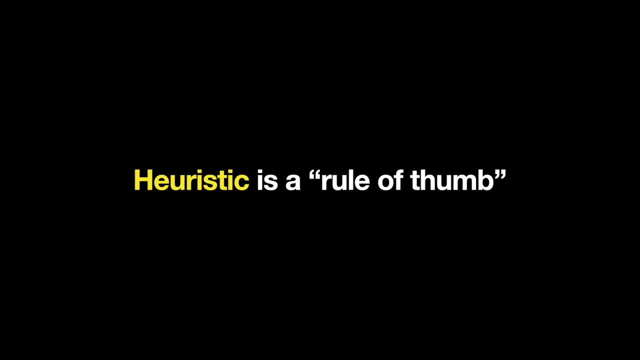 The word heuristic means a rule of thumb. A heuristic is a very general rule or principle that applies to a wide range of user interfaces. When we talk about heuristic evaluation, we mean using a list of heuristics to check if the products satisfy them. 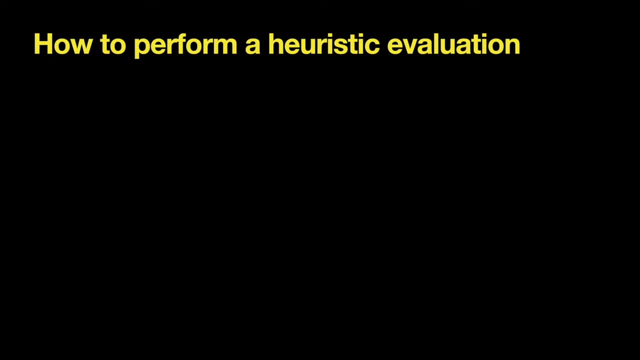 Here is how to perform a heuristic evaluation. First, you need to define a scope. Doing a heuristic evaluation of an entire product isn't a good idea, especially when working on a large-scale product. Heuristic evaluation of the entire product could take a long time. 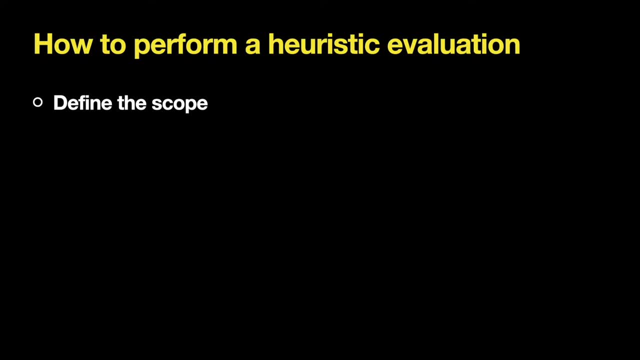 and become very expensive. That's why it's recommended to conduct a highly focused heuristic evaluation, Focus only on the most critical areas of the product. Next, you need to invite usability experts. Usability experts are professionals who can evaluate your user interface and accurately judge what will irritate users. 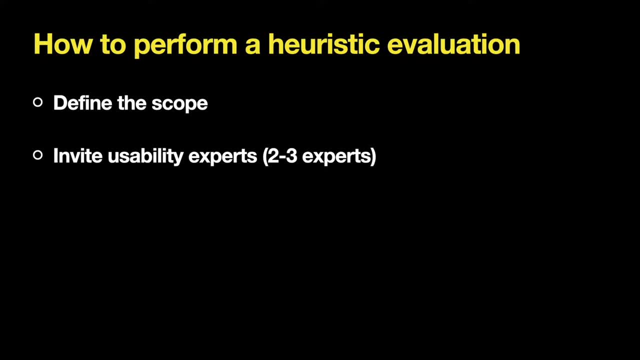 Usability experts don't need to be users of your product. Ideally, you should invite three experts who can define the evaluation criteria and assess your products against it. If you invite more than three experts, you will likely see a sharp reduction in evaluation results. 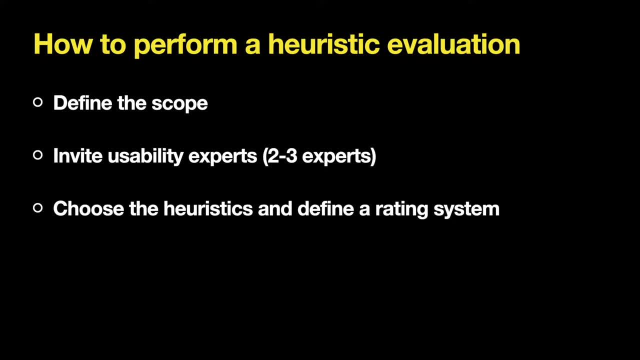 Heuristic. evaluations rely heavily on the heuristics that are defined or chosen Together with experts. you need to choose heuristics that you will use to evaluate your product. Experts should know exactly what they are supposed to do during the evaluation, So it's recommended to hold a briefing session during which you will ensure that experts receive the same instruction. 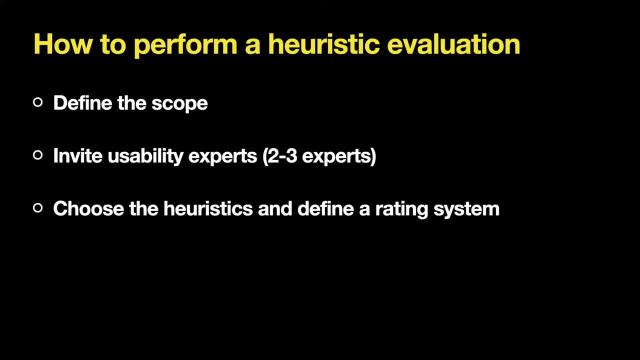 Most experts use between 5 and 10 heuristics when they do evaluation. The heuristics should be chosen based on their relevance to the product that is being tested. A rating system will help you prioritize the list of usability issues found by the experts. 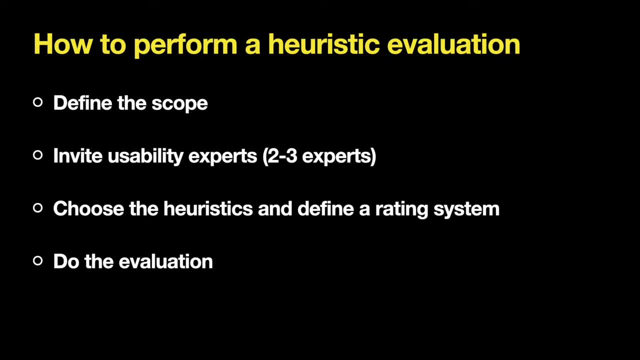 Next, do the evaluation. Ensure that all experts use the same set of heuristics and do assessments independently. It will help you receive unbiased results At the end of the heuristic evaluation. it's essential to aggregate the heuristic evaluation reports from usability experts. 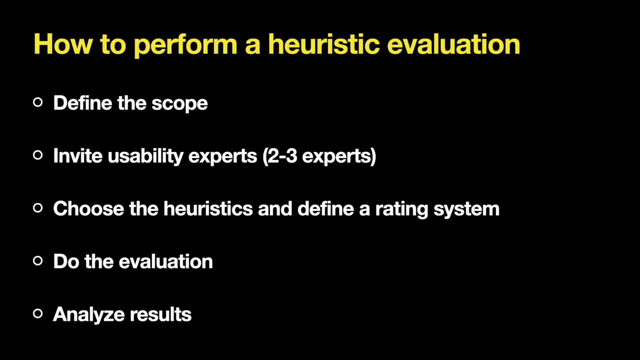 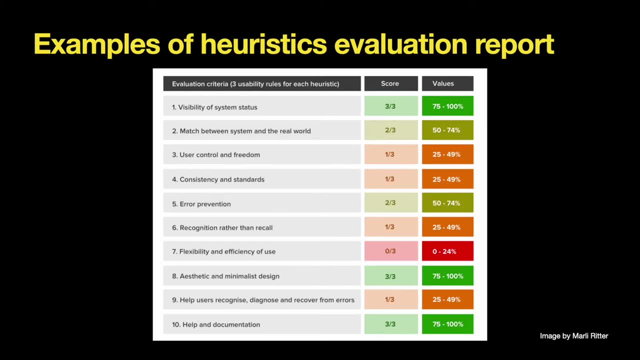 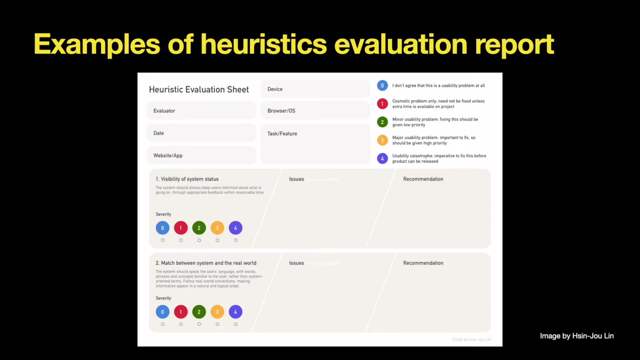 And build a list of usability issues that needs to be fixed. Here is the first example of the heuristic evaluation report. It shows the scope compared to how many rules were followed for each heuristic. And here is another example of the heuristic evaluation report. It shows the severity of the issues and provides recommendations on how to solve them. 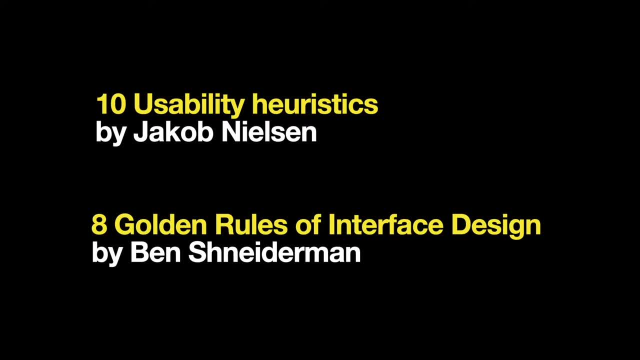 Jacob Nielsen's 10 usability heuristics for user interface design and Ben Schneiderman's 8 golden rules of interface design are probably the most commonly used set of usability heuristics. In this video I will cover Jacob Nielsen's 10 usability heuristics. 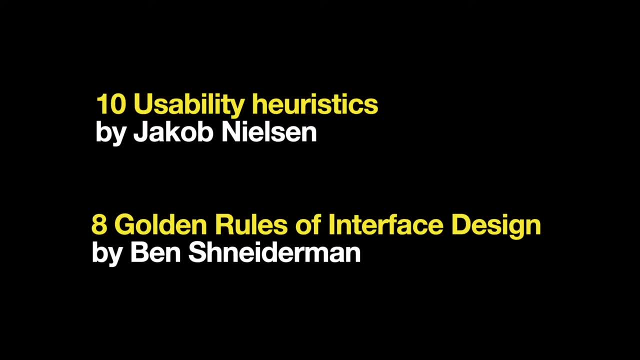 The great thing about the set created by Jacob Nielsen is that it remains the same since the moment he defined it in 1994.. And it's likely the heuristics will be relevant for the future types of heuristics. That's because heuristics come from the basic understanding of human psychology and the way people interact with the product. 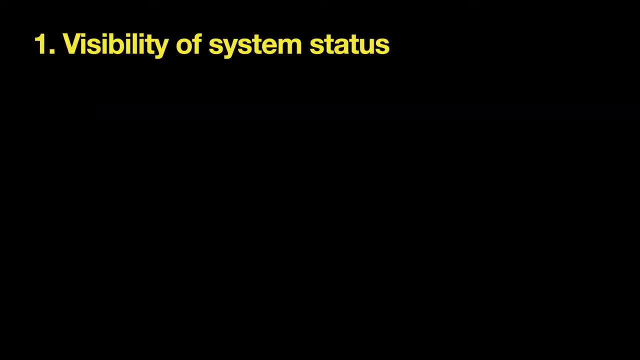 Let me walk you through each of the heuristics. The first heuristic is the visibility of a system status. This system should always keep the user informed about what's happening. When you design a product, you shouldn't make the user wonder what's happening. 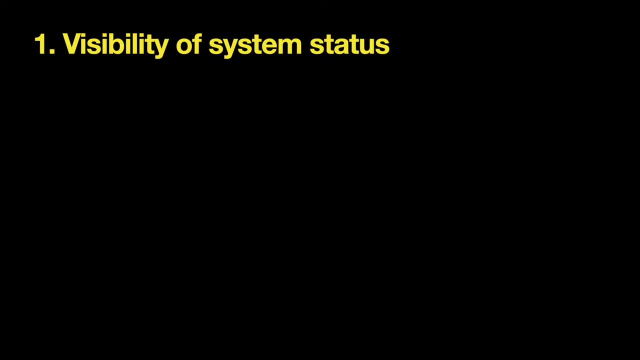 Or offer any sort of feedback- Visual audio haptic- to help the user understand the current status. It's particularly important to provide feedback on actions initiated by the user. In such case, the feedback acts as acknowledgement for the user. Users understand that the system received their request and working on it. 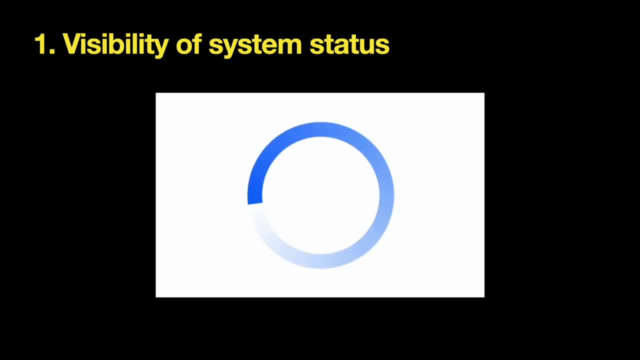 Loading is one of the cases when you need to inform the users about the current status. Load time can vary drastically depending on the context, And when users don't have any feedback, they simply don't have any information whether the system is doing something or not. 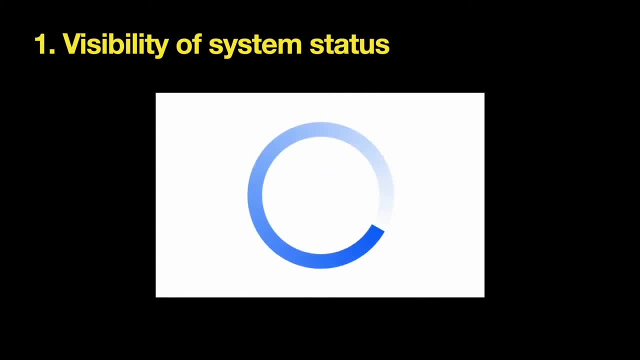 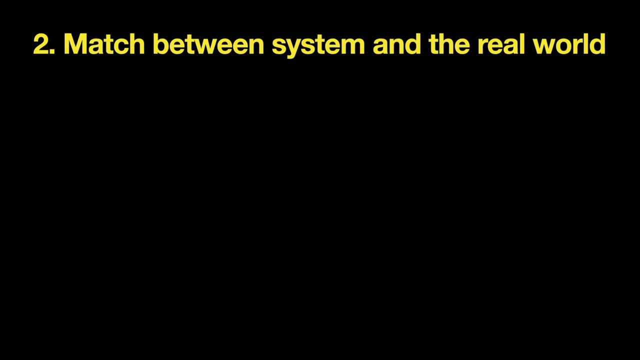 Feedback alleviates any fears that the system is not responding. Match between system and the real world. The system should use language that is easy for your users to understand. It means that the terminology as well as the concept and metaphors used in the digital products. 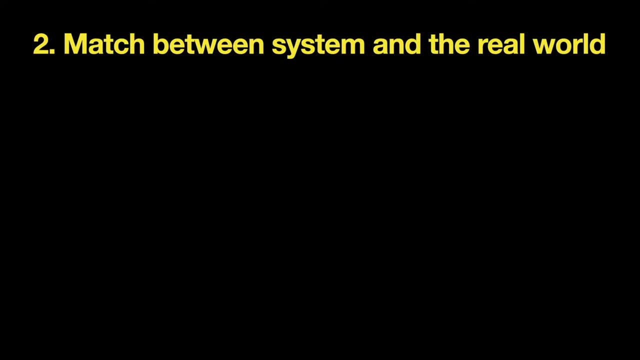 should be natural to your users. It's essential to identify all places in your app that can cause confusion and redesign them to make them evident for your target audience. Confusion can be caused by unfamiliar terms or unfamiliar concepts. To beat the first problem, you need to avoid jargon and use terms that are familiar to your target audience. 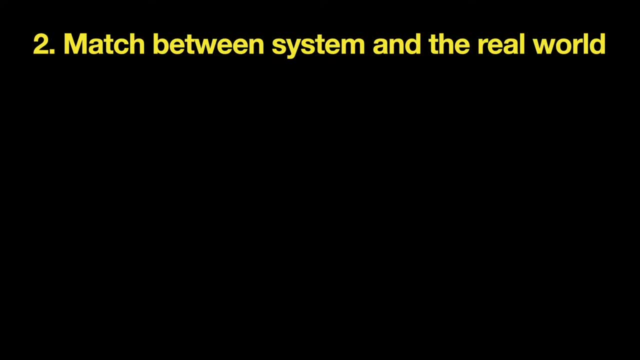 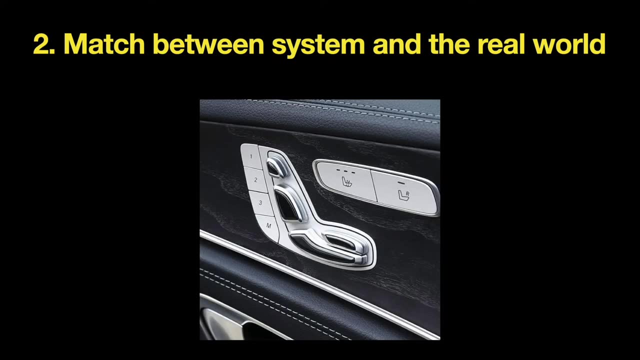 To overcome the second problem, you need to rely on analogies from the real world. Here is a nice example of design that follows this rule: Mercedes uses a metaphor of a physical chair for their power seat adjustment controls. It helps passengers to understand how to adjust the seat according to their needs. 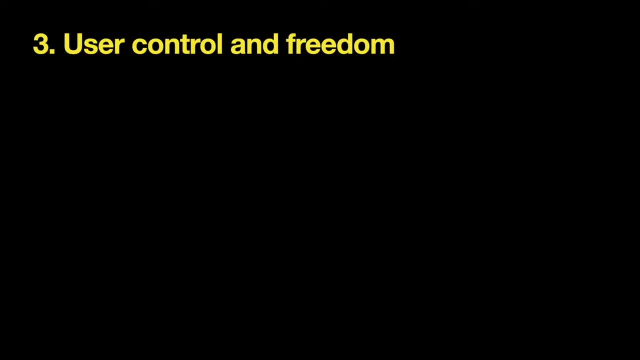 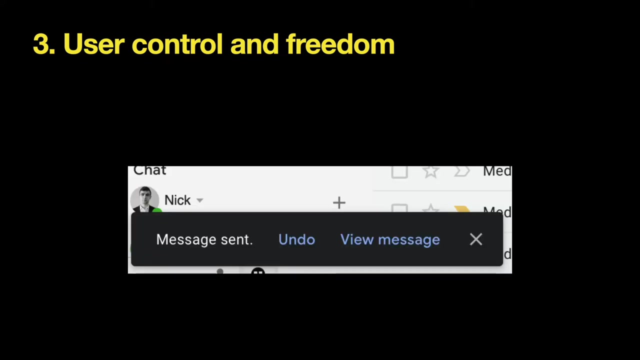 Third, user control and freedom. The system should offer an emergency exit because people make mistakes when they interact with the product. Users should be able to undo and redo actions. When users send a message using Gmail, the service offers a confirmation dialog with the undo button. 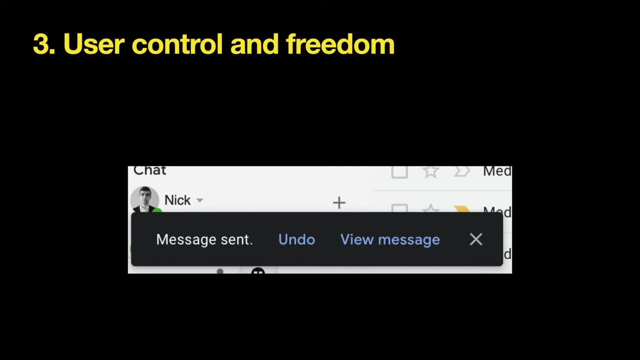 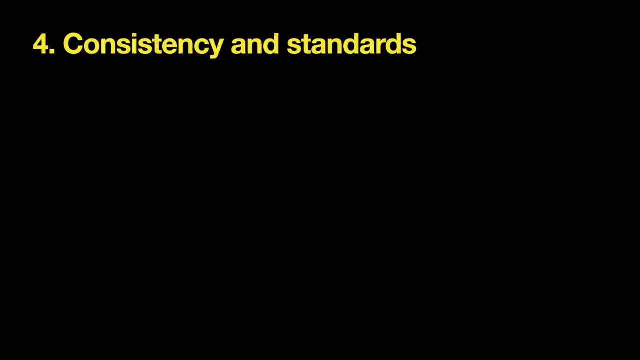 The undo button allows users to cancel the sending if the message was sent by accident. Consistency and standards. Users shouldn't have to worry whether the different words, situations or actions mean the same thing. Designers should strive for a consistent design. 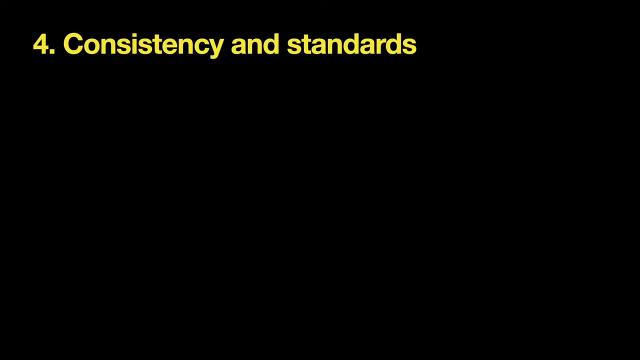 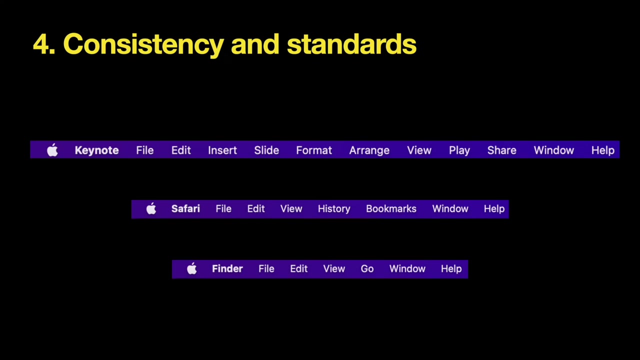 They have to offer internal consistency and external consistency. The location and design of navigation menu in Apple Mac OS is consistent. Both the order of the navigation options and their visual appearance is the same. in general, There is no need to worry about the layout of the navigation menu. 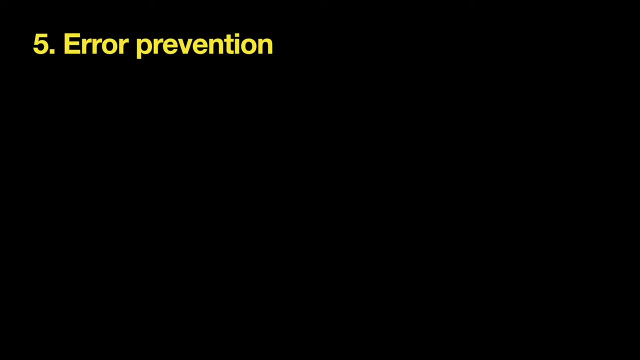 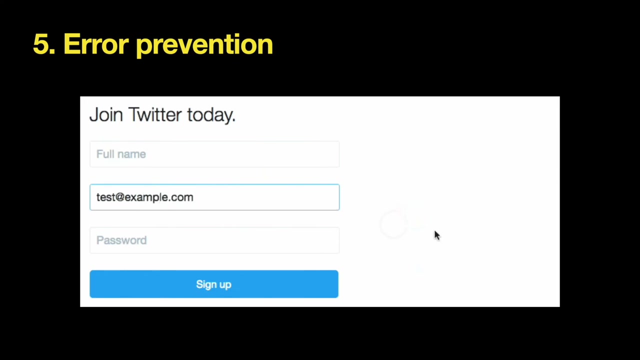 Error prevention. Errors should be kept to a minimum. Prevent errors from happening by designing for situations where users might face problems. You need to design your products to minimize the total number of cases when users can face problems and will need support and assistance. For example, when a user provides input. you can use inline validation. 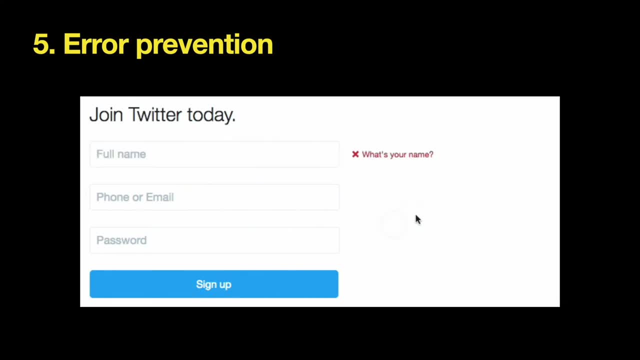 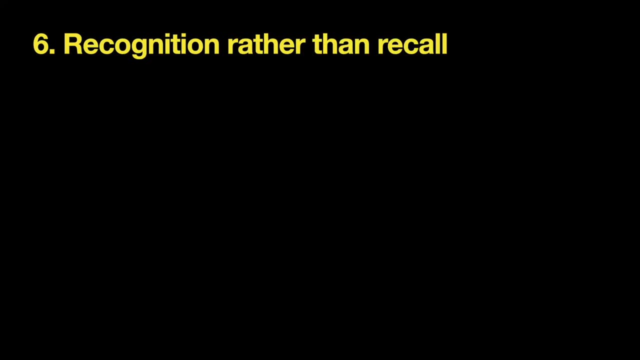 To validate the data on the fly, So the user don't need to tap the submit button. Recognition rather than recall: Humans can recognize things much more easily than recalling them from scratch. Product designers should minimize the user's memory load by making objects, actions and other options visible and clearly communicated. 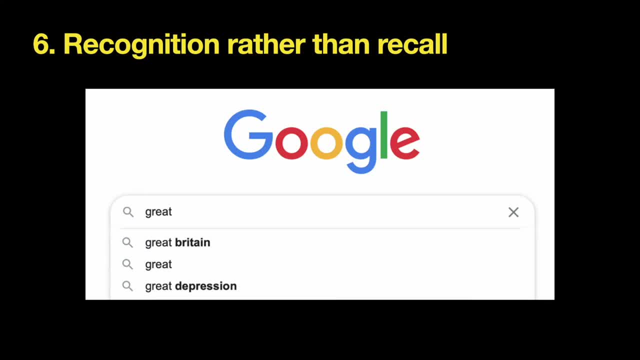 Don't make users worry. Provide all required suggestions at the moment when users need them. Contextual recommendations in Google Search is an excellent example of recognition rather than recall. As the user starts typing, Google Search suggests the relevant queries, And this helps users find the right query in less time. 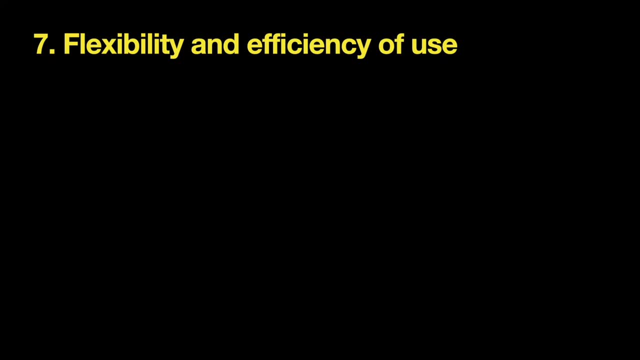 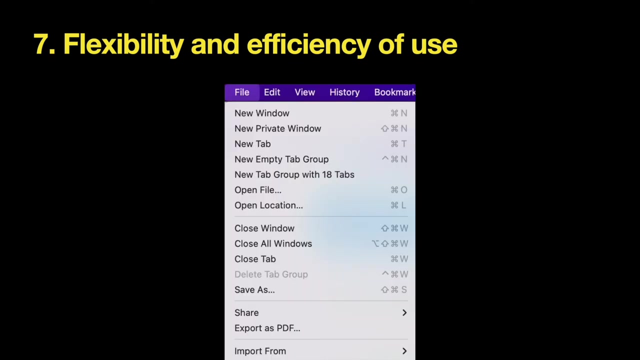 Flexibility and efficiency of use. Accommodate both novice and advanced users, But tailor the experience for both groups. Provide ways of speeding up workflows and accelerating users familiar with the system While guiding those who are less familiar. For example, you can offer shortcuts that can speed up the interaction for the expert users. 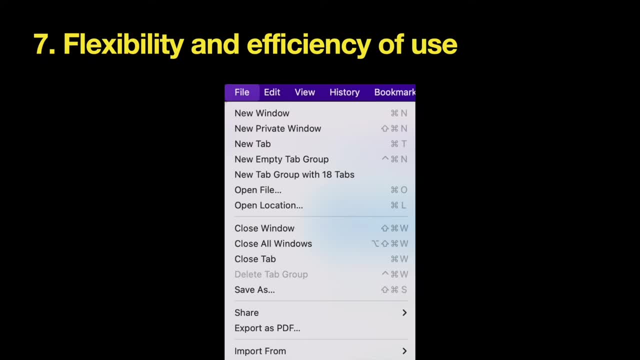 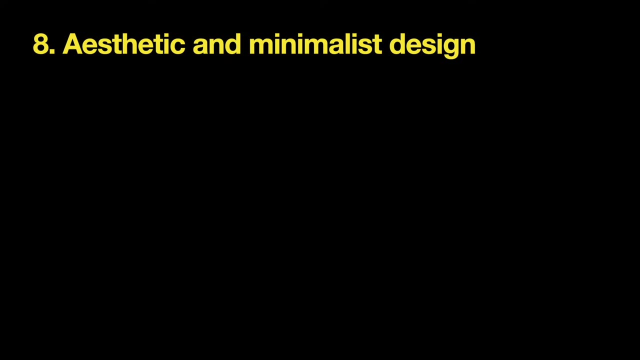 Keyboard shortcuts are available in many products And they enable users to use frequent actions without clicking the button In the menu. Iaesthetic and minimalism: Follow the less is more approach in your design. Remove all unnecessary elements that do not have any positive impact on the user experience. 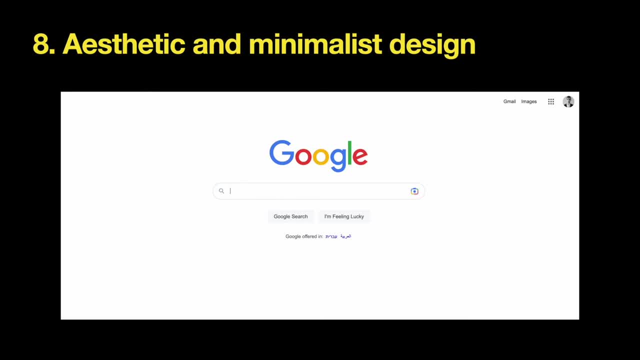 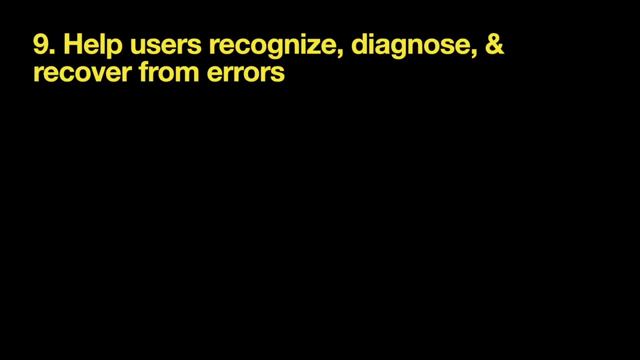 Google Search is an excellent example on how to prioritize content over Chrome. The service removes all unnecessary visual design details And the page is centered around one particular idea. Search Help users recognize and recover from errors. Error messages should be expressed in a plain language. 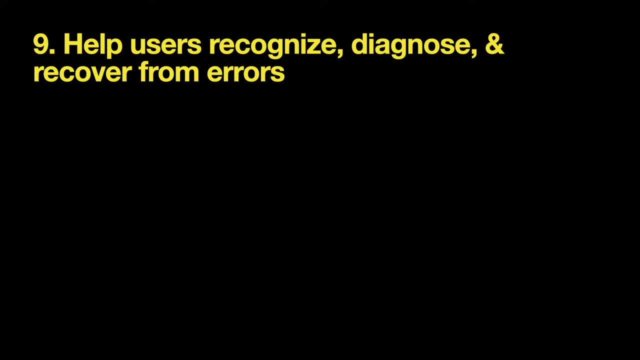 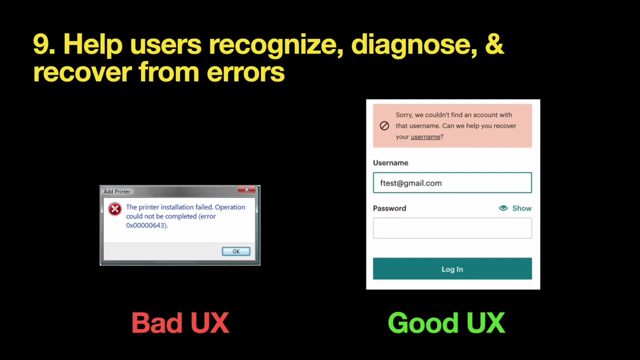 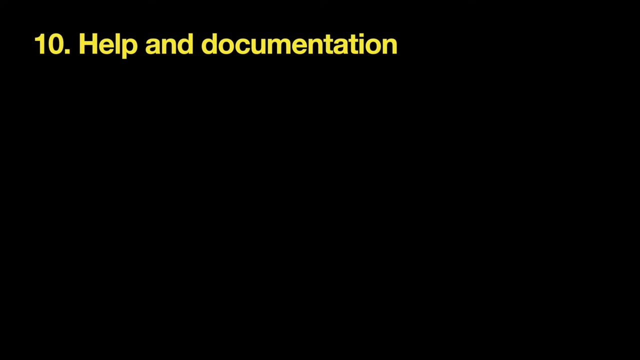 Precisely indicate the problem and suggest a solution. When writing error messages, do not only state the fact that users face a problem. Offer a solution on how to solve it. Help and documentation: Offer helpful documentation inside your product. Documentation should be a natural part of your product. 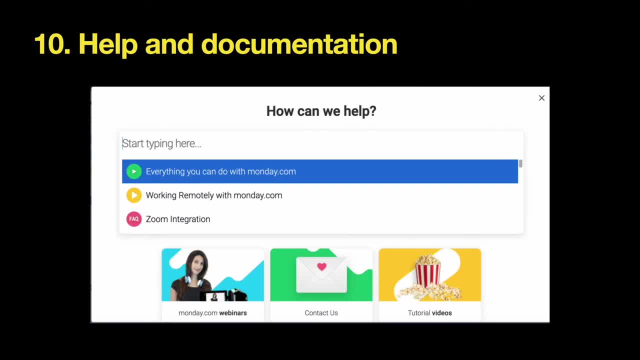 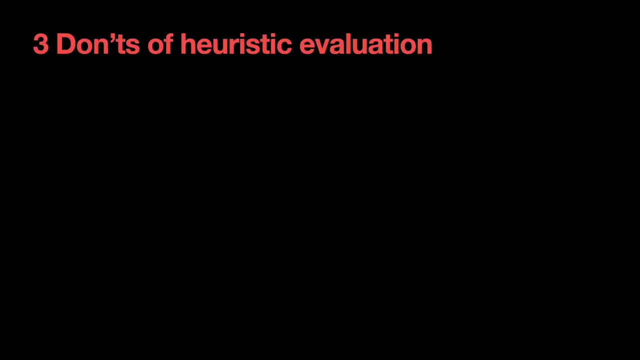 And it should be refined regularly. Always think about specific situations that a user can face Or questions that a user might ask while they interact with your product, And cover them in the documentation. Now let's talk about things you shouldn't do when conducting heuristic evaluation. 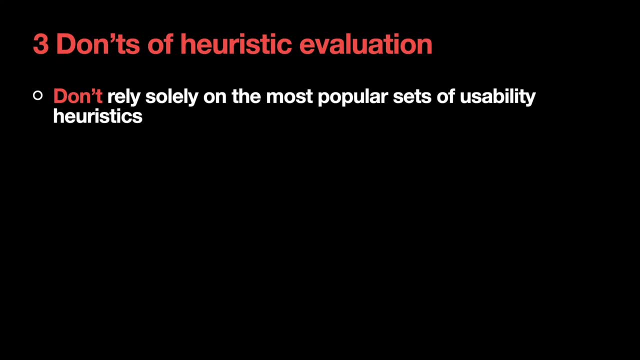 First, don't rely solely on the popular heuristics When it comes to establishing design heuristics. there are no fixed recommendations, as each design presents its own set of different needs. The heuristic coined by Jacob Nielsen or Ben Schneiderman should be used to inform usability experts.